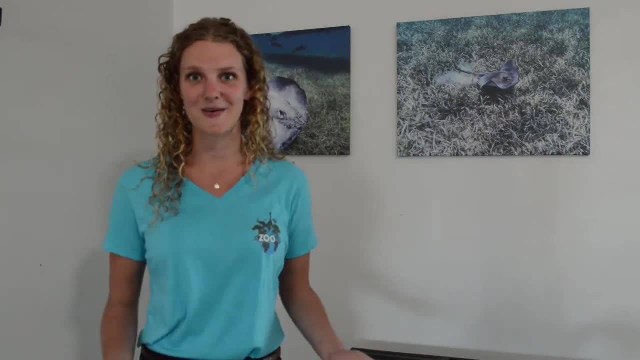 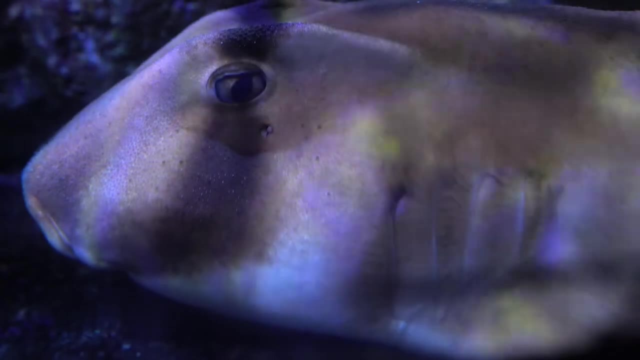 are lots of animals that live in the ocean. The most obvious one is fish, And they are very special for the ocean because of their gills. right, Those gills help pull oxygen out of the water and allow them to breathe, without having to come up to the surface of the water to get a breath of. 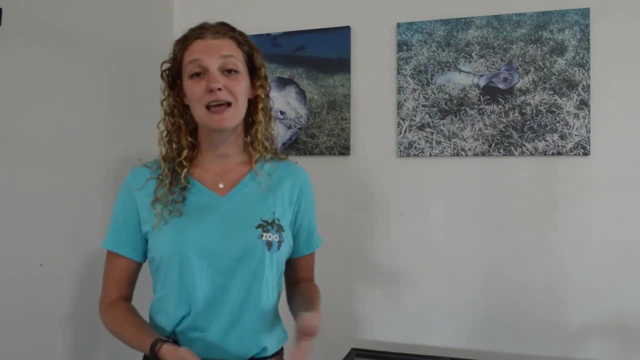 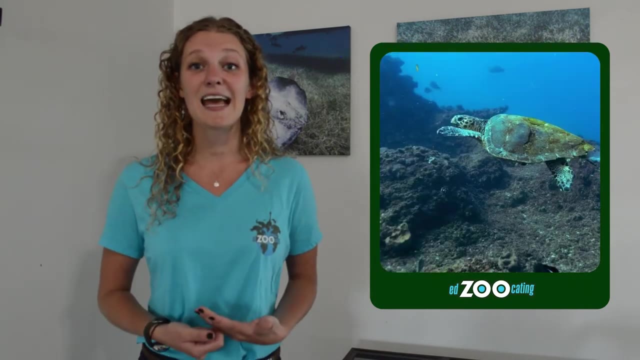 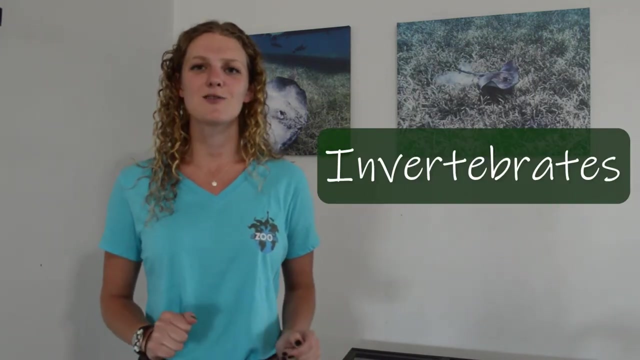 air, But we find more than just fish in the ocean. We can find mammals like whales and dolphins. We also find reptiles like sea turtles, And there are lots of invertebrates in the ocean, And invertebrates are animals that don't have any bones. So this is going to 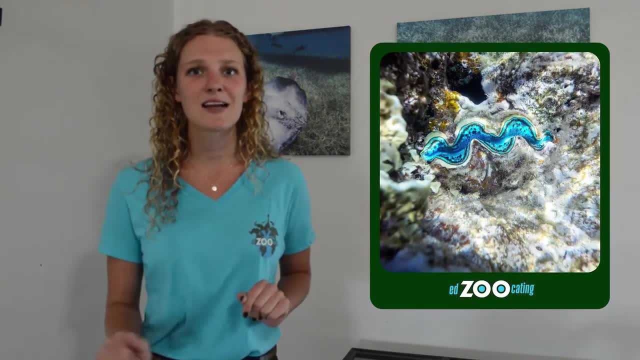 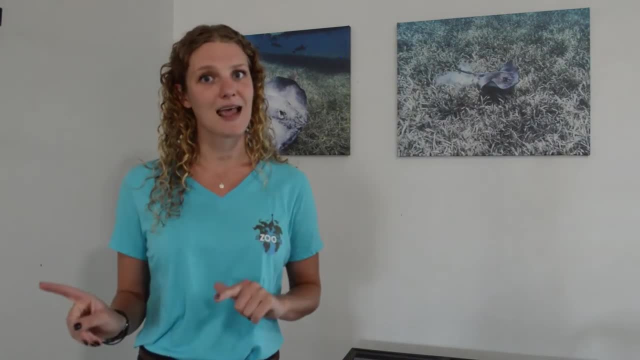 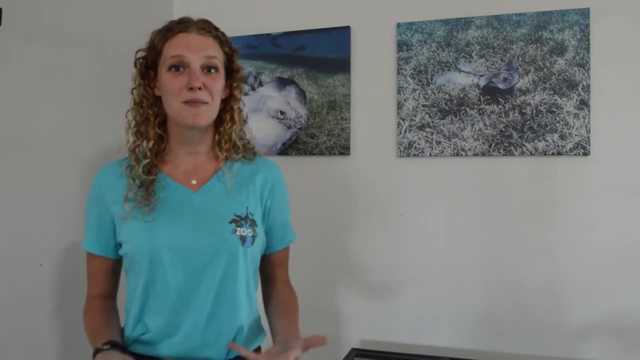 be animals like sea stars and sea urchin, clams and crabs- all sorts of different animals that call the ocean home. Biotic factors can also be plants, So we might think of a plant like seagrass, which you guys can see behind me. Seagrass is a really yummy meal for animals. 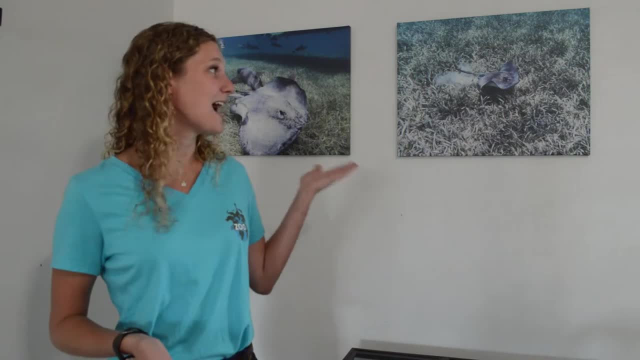 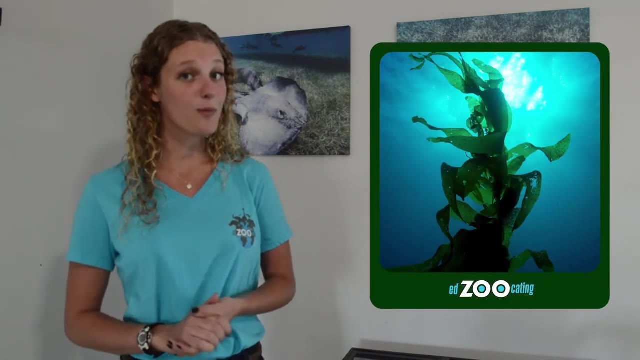 like sea turtles and manatees, But it's also a great hiding spot for stingrays, just like you see here. They love to hang out in the seagrasses. We also find kelp, which we're going to be talking about in a little bit. So we're going to be talking about kelp, which we're going to be. 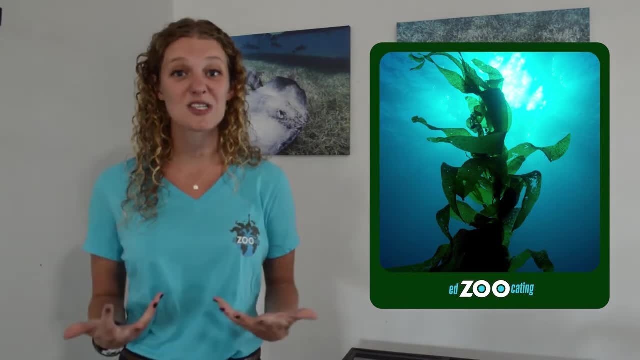 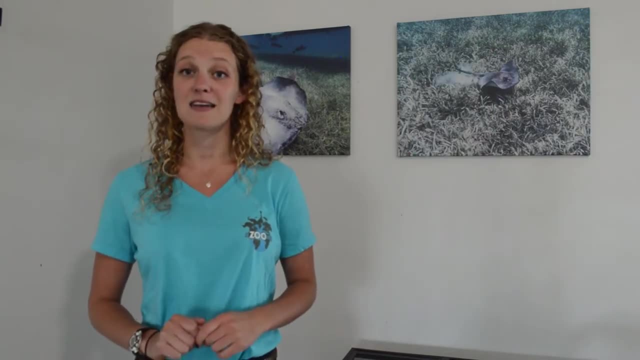 talking about more in just a little bit. Kelp is one of the largest and fastest growing plants in the entire world, But perhaps the most important plant that we find in the ocean is one that a lot of times we can't even see, We don't even know it's there And we call this plant. 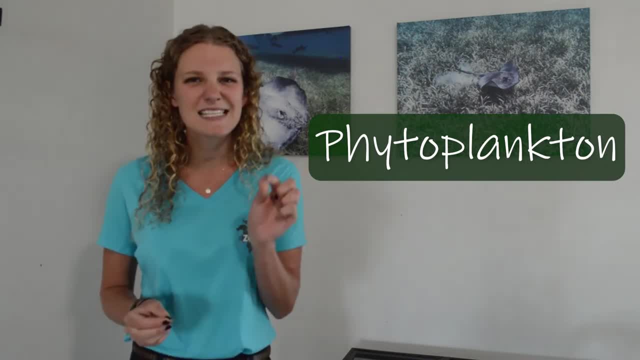 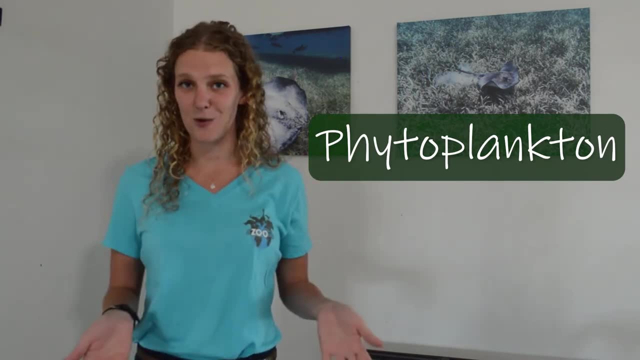 phytoplankton. Phytoplankton are teeny, tiny, little microscopic plants that float around near the surface of the ocean where the sun shines down and they can photosynthesize. And phytoplankton are super important because of the amount of oxygen it produces. It produces some scientists. 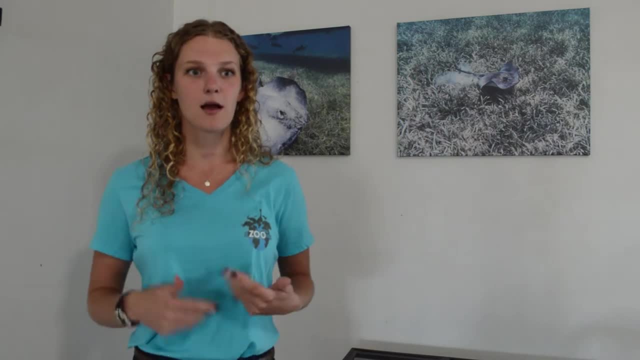 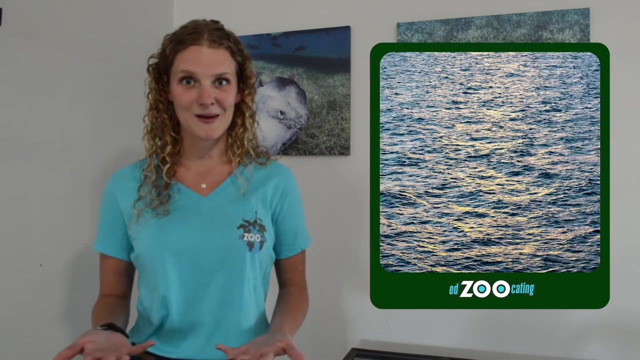 think more than half of the oxygen that's in our atmosphere comes from tiny little plants floating around in the ocean. So now we've talked about the biotic factors, but let's think of some of the abiotic factors. Obviously, the biggest abiotic factor is saltwater. The ocean is filled. 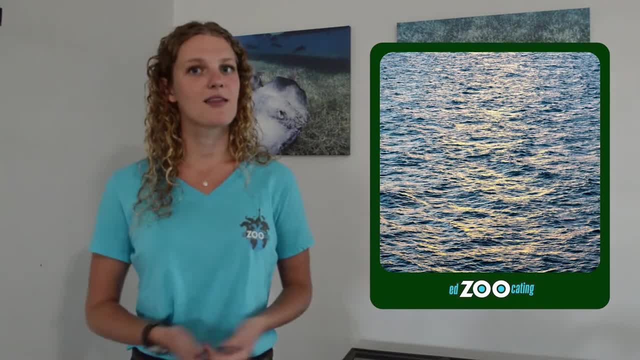 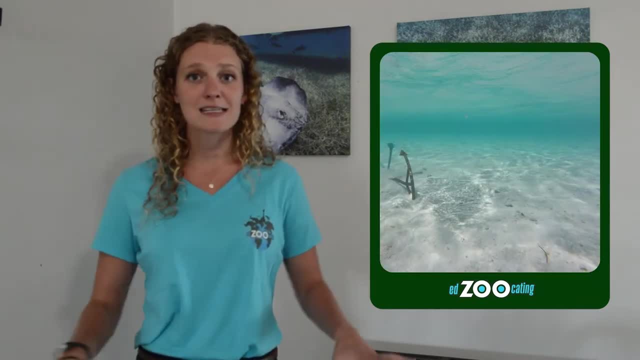 with saltwater, which is not living, but there are lots of other abiotic factors that are living in the ocean. So we can think of the ocean as a place where we have a lot of oxygen, but there's also a lot of rocks down there mixed about. Also, the ocean is filled with lots of different temperatures. 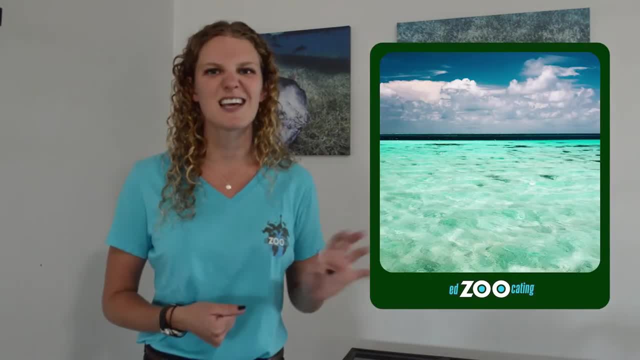 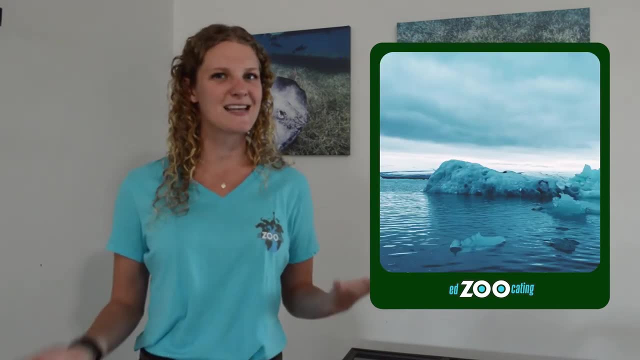 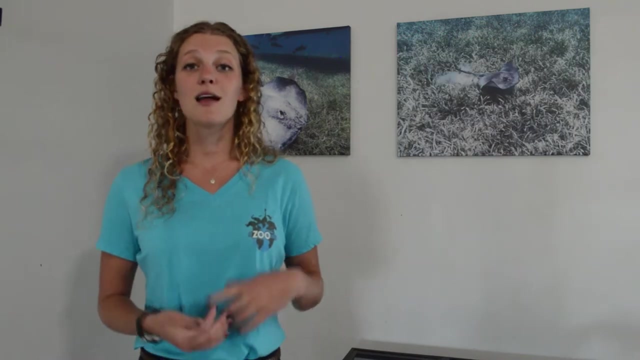 So just like we think of tropical oceans that are nice and warm, we can think of oceans that are up by the North and South Pole that are freezing cold. So, depending on where we are in the ocean, these abiotic factors can be really different from one another. So not only is the ocean, 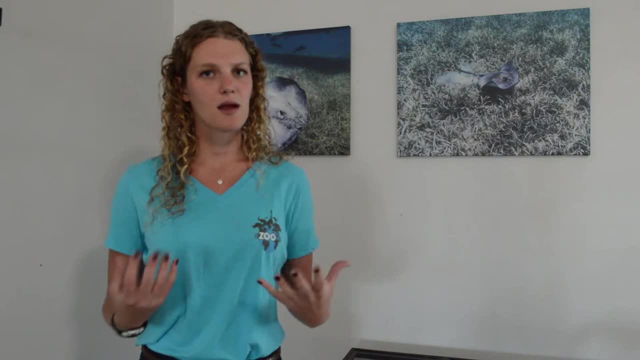 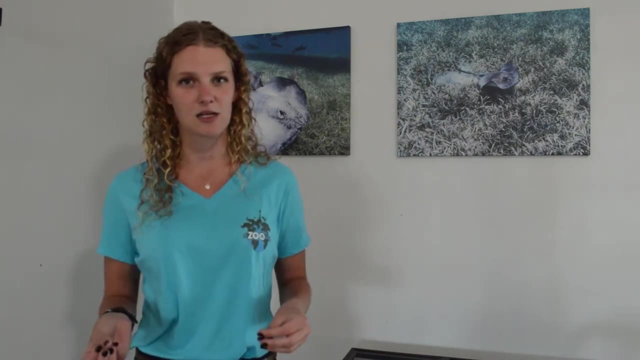 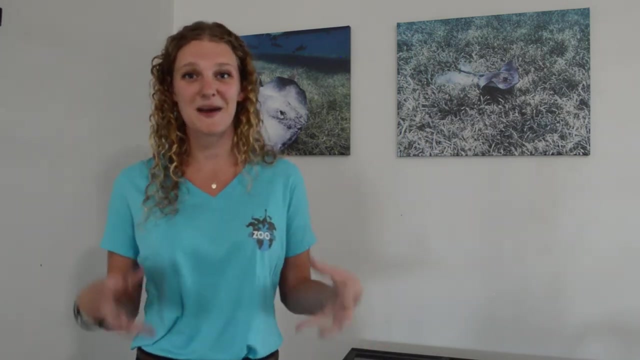 filled with biotic and abiotic factors. but, like we just said, different parts of the ocean are home to different types of organisms and different types of abiotic factors. So let's spend a couple minutes and talk about some of these different habitats, some of these smaller areas in the ocean. 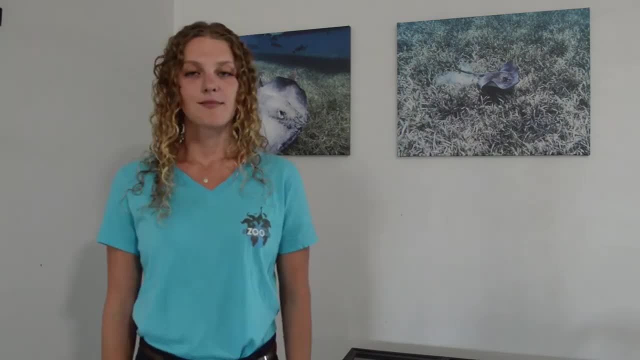 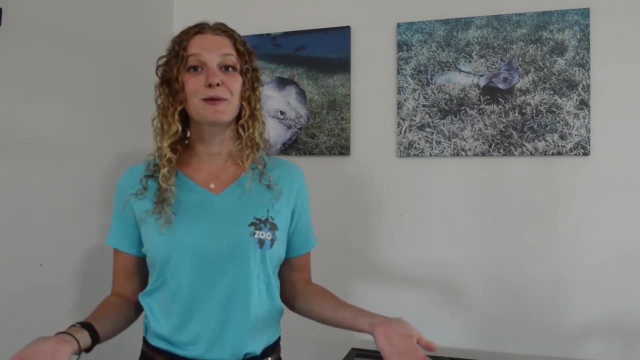 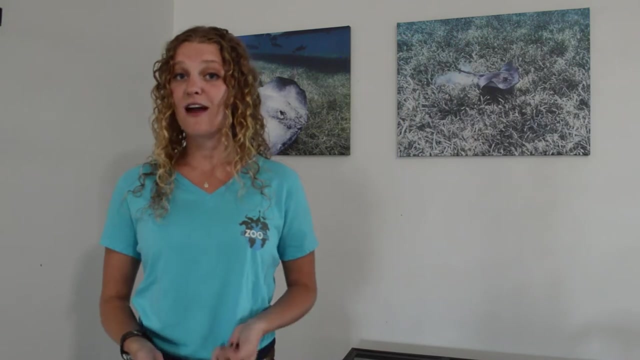 that lots of different plants and animals call home. Let's start off with a coral reef. I'm sure a lot of you guys are familiar with coral reefs, because this is where we find a lot of different animals, And coral reefs are found in warm and shallow waters, which makes a really great place. 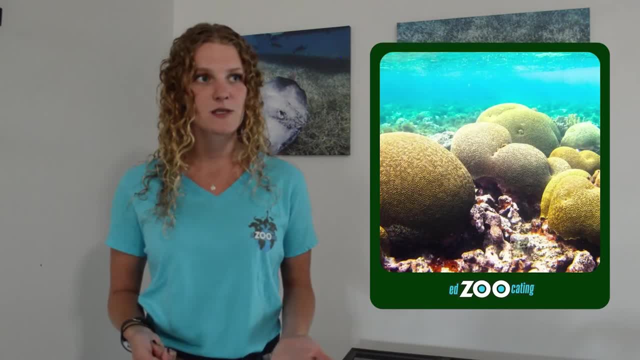 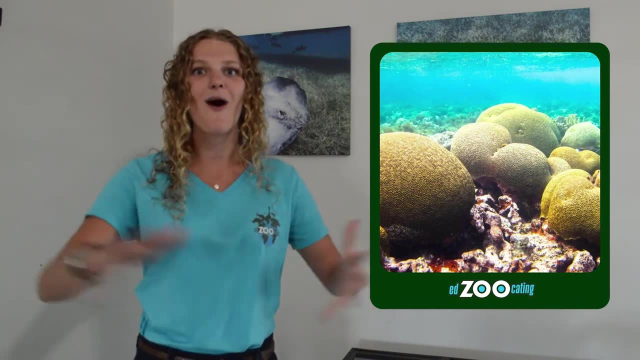 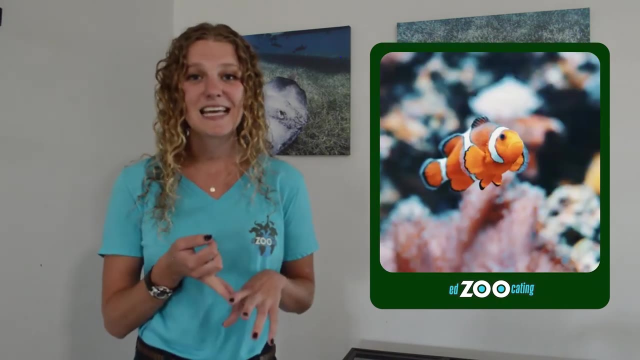 for animals to live, And the corals themselves are actually animals as well. They're teeny, tiny, little animals that work together to create corals, And then all of the corals create these big coral reefs, And coral reefs are home to animals like little fish and eels, lots of. 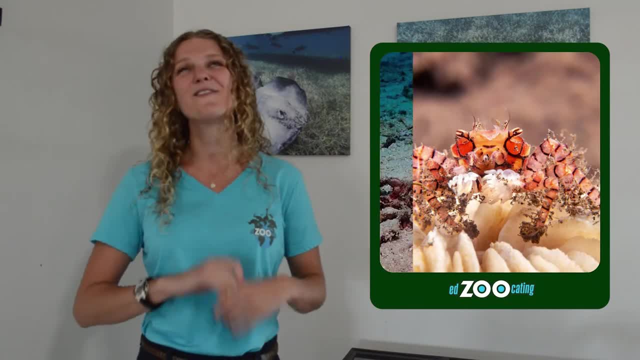 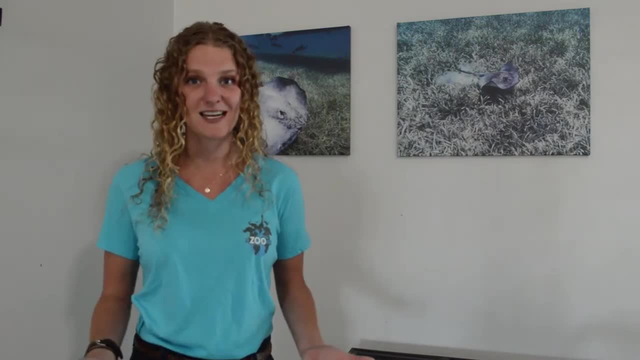 crustaceans and a lot of other animals. So corals are home to a lot of different kinds of animals, Like crabs, sea snakes. We find tons of little animals hanging out in coral reefs because there is lots of protection. So, because there's so much protection and so many little things growing, 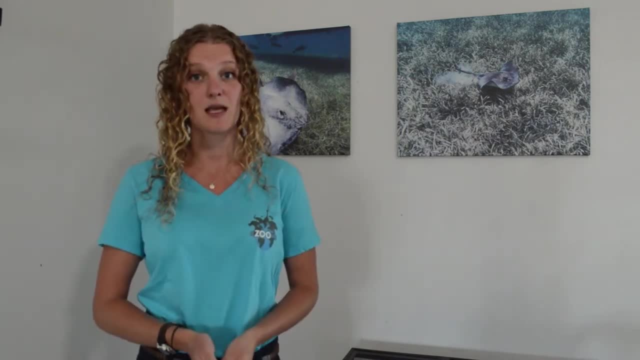 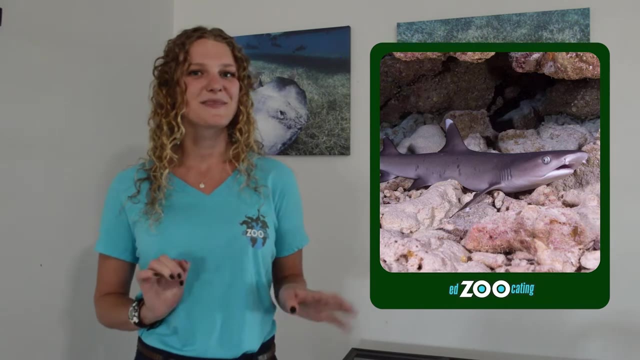 around. there's lots of good resources for little animals, But we also find big animals in coral reef. We find sharks, which come into the coral reefs especially at nighttime, looking for little fish that haven't quite been hiding yet. We also find sea turtles, which are really big animals. 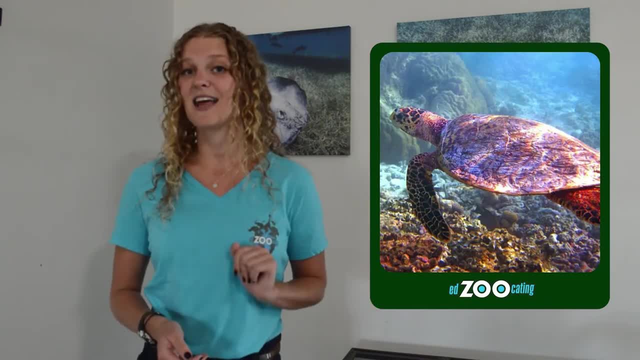 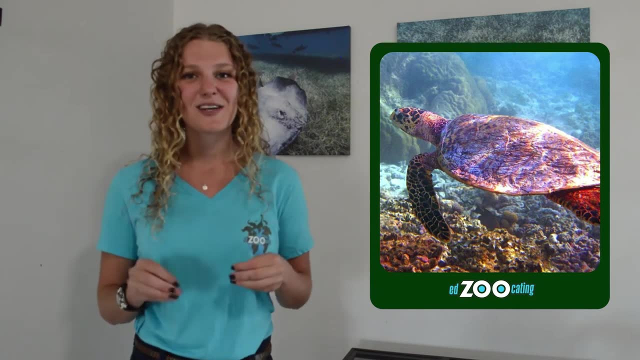 We also find sea turtles, which are really big animals. We also find sea turtles, which are really turtles, who come into coral reefs. A lot of the times they are looking for a little shrimp called a cleaner shrimp that will hop right up onto their backs and eat any algae or any parasites that. 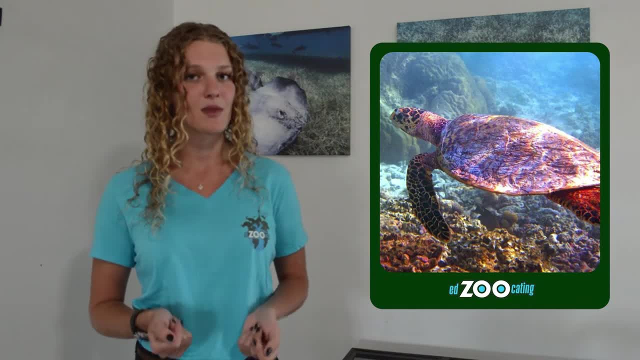 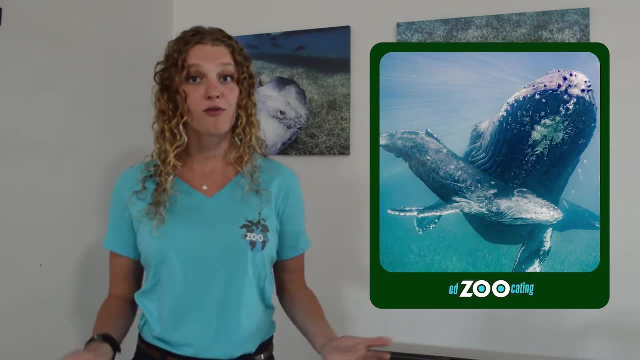 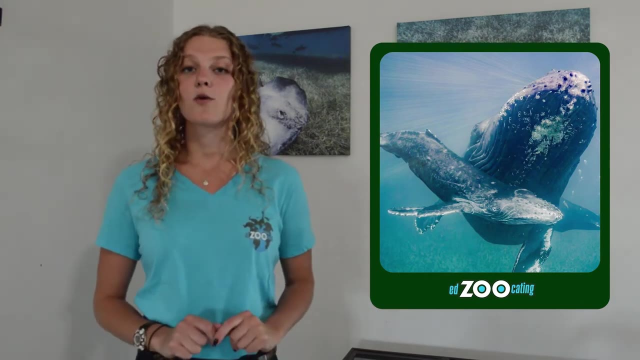 might be growing on their backs and helps kind of keep them clean. We also find whales sometimes near coral reefs. Because of all of the protection a coral reef provides, that's a really great spot for whales to go and have their babies, somewhere where it's nice and safe. So coral reefs are. 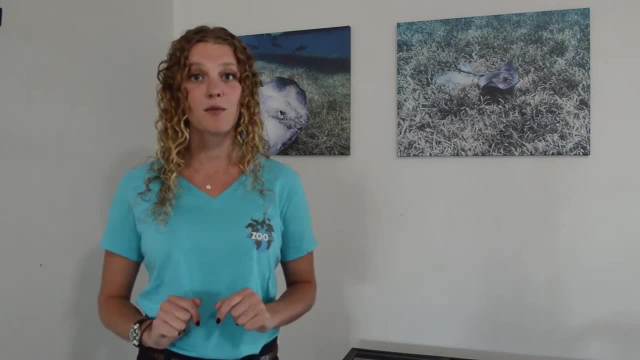 home to a ton of different plants and animals. We actually call coral reefs rainforests of the sea because so many plants and animals live there. Scientists think more than 25% of all marine life calls the coral reef home at some point during their lives- Another ocean habitat that provides 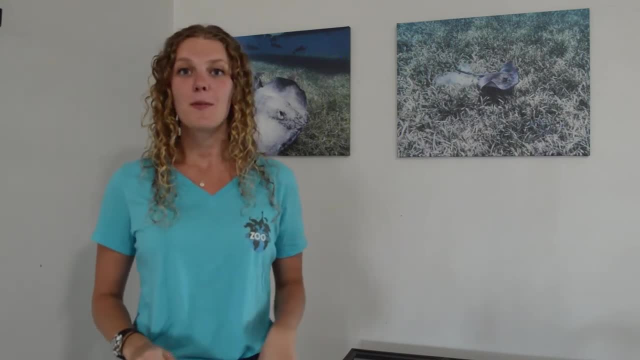 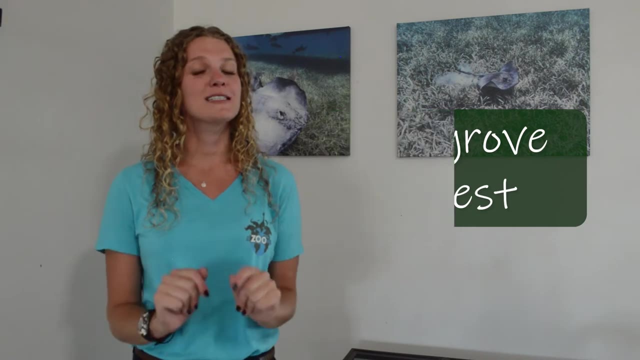 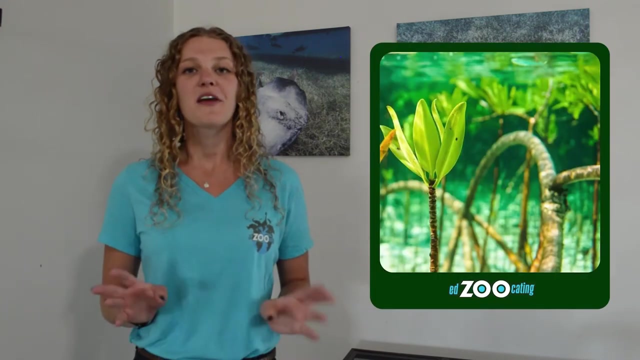 lots of protection, just like a coral reef, but is not quite as well known as a coral reef is the mangrove forests, And mangrove forests are even a little bit cooler than a coral reef, because not only do they provide protection underwater, but they also provide protection above the water. So 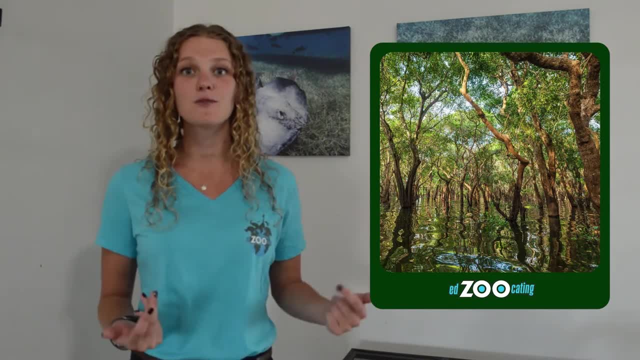 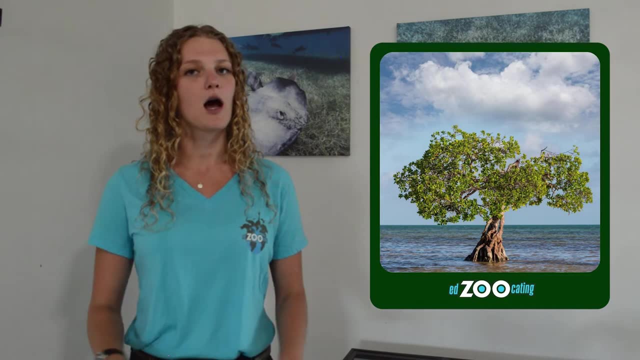 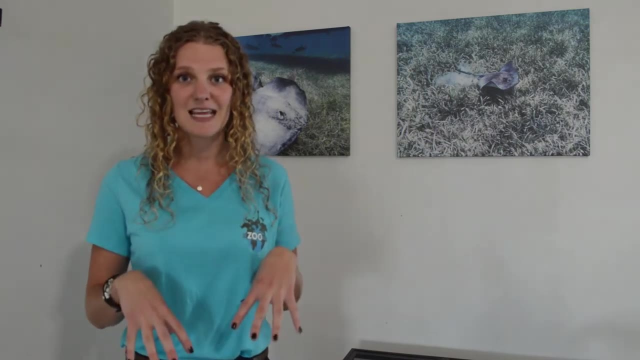 a mangrove forest is made of very special types of trees, like the name forest suggests. And these trees are really special because their roots are not under the sand like other aquatic plants. Instead, their roots are actually above the sand And then the branches are above the water, So beneath the water, where all of those 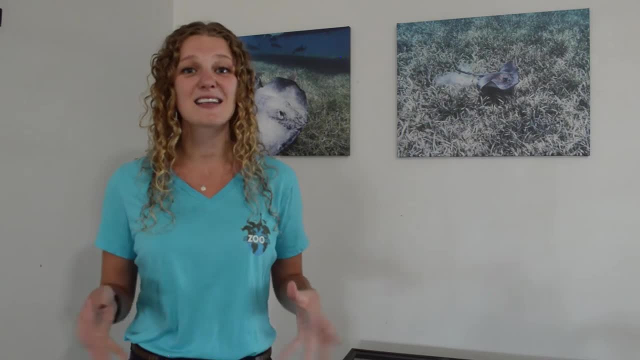 roots are. there are tunnels and hiding spaces that lots of little fish call home, And so do crabs, And mangrove forests are, a lot of the times, a nursery for bigger fish. When they have young fish who are really easy prey, they can hang out in these mangrove forests where there's a little. 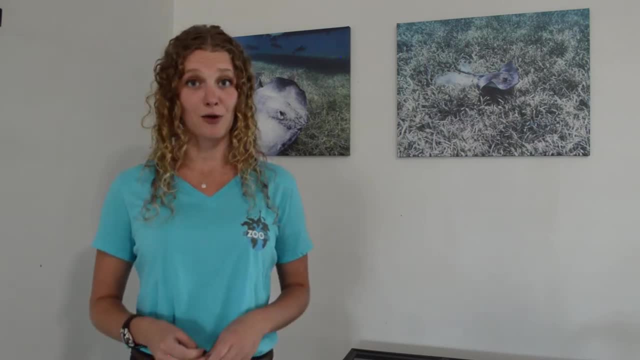 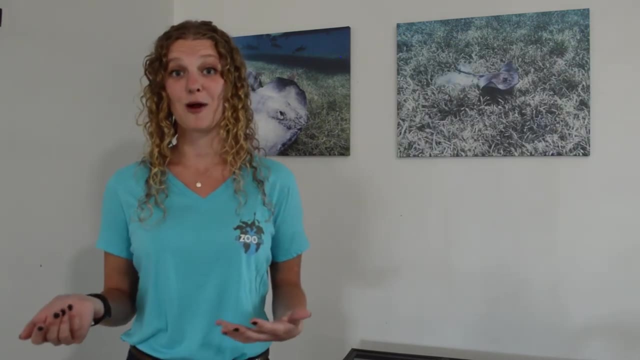 bit more protection And we find lots of different invertebrates in a mangrove forest. So mangrove forest, So lots of different types of snails. We even find reptiles hanging out in a mangrove forest, But usually the reptiles are up in the branches. This is where we might find snakes. 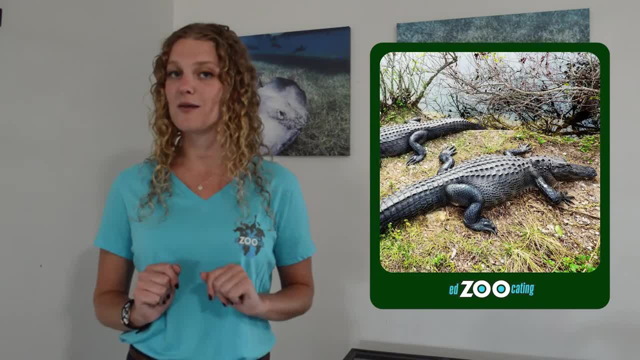 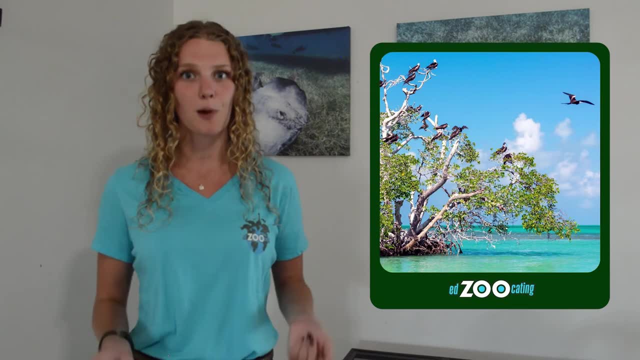 Lots of different snakes, even alligators, will hang out in a mangrove forest above the water, where they also have protection, And lots of different types of birds also hang out in a mangrove. That is a great place for them to hunt all of those little fish that I'm talking about. 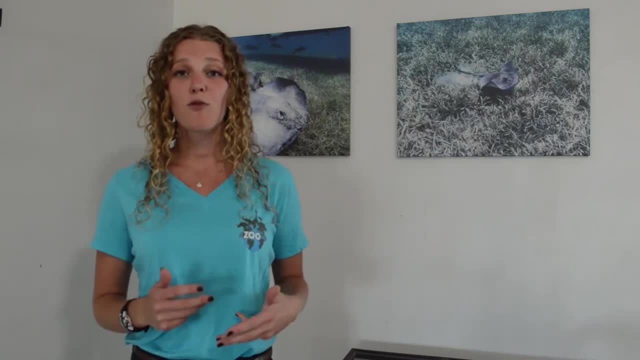 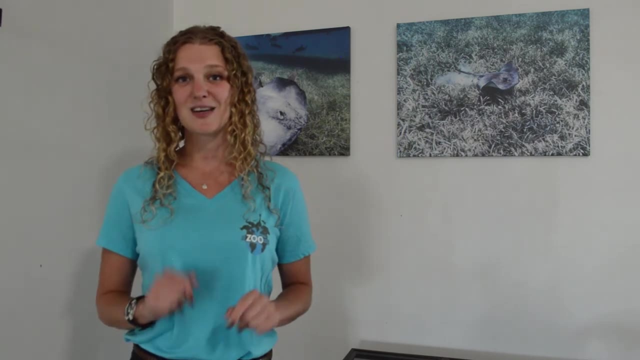 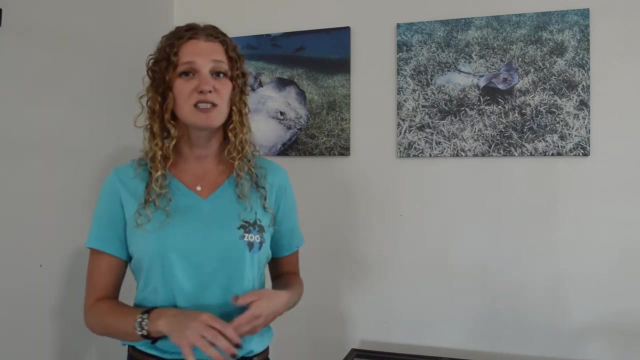 So mangrove forests are also found in tropical regions. So the waters are a little bit warmer, the air is a little bit warmer too and there's lots of sunlight, But mangrove forests lots of times have flooding, where the water goes in and out. So lots of abiotic factors that cause a. 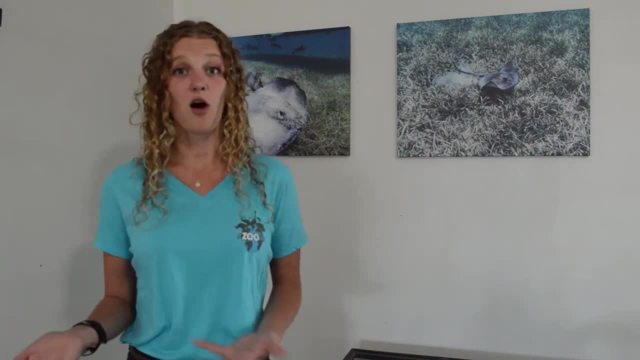 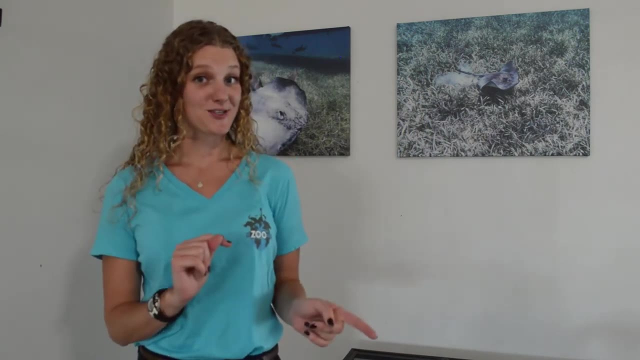 little bit of challenges to all of these plants and animals that live in the mangrove forest. So now, if we move just off of the shore, we're going to see a little bit more of the mangrove forest. We might find ecosystems like kelp forests, And kelp forests are found in warmer waters. 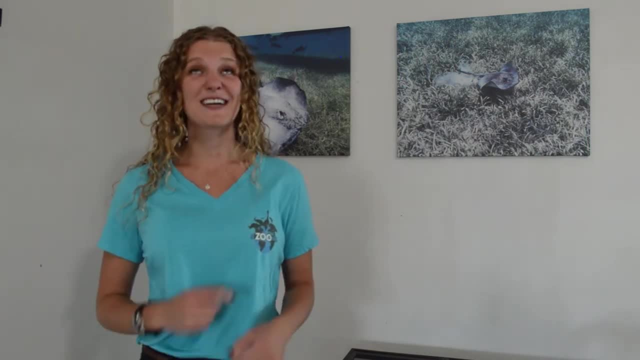 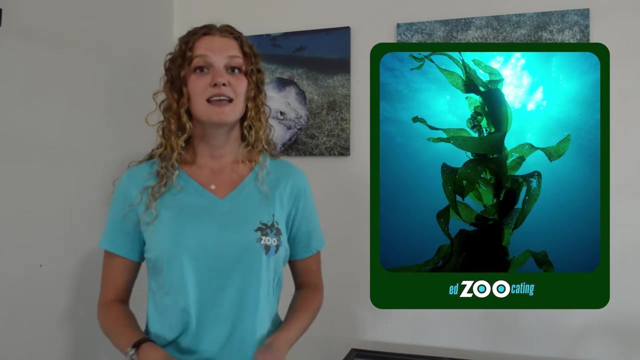 but they're also found in colder waters, which means that there are a ton of different plants and animals that can tolerate both warm and cold water. So that again is one of those abiotic challenges that plants and animals face. And we mentioned kelp before, because kelp is one of the 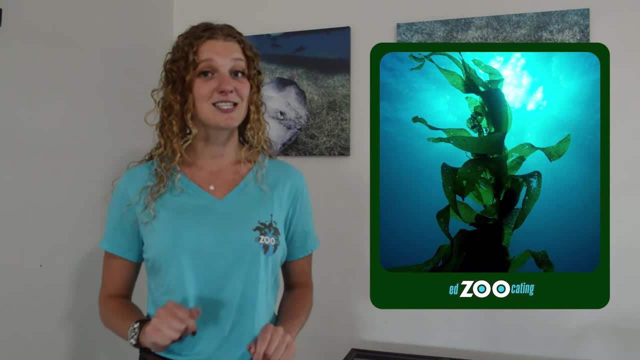 fastest growing plants in the world. In the right conditions, they can grow almost two feet per year, And they can grow up to two feet per year, And they can grow up to two feet per day, which means that there's lots of plants and lots of good hiding spaces for animals, So of 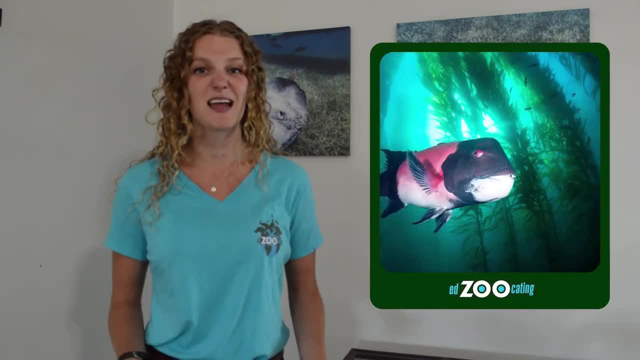 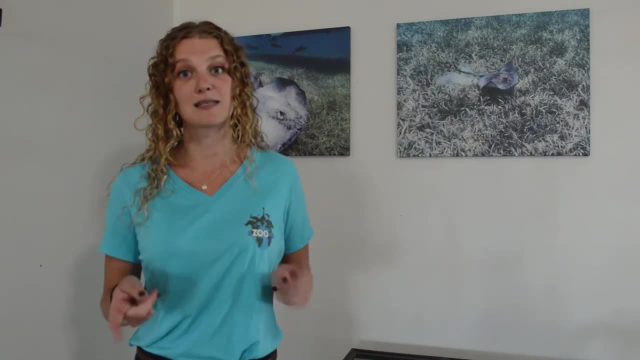 course, in a kelp forest we find lots of different types of fish and we find sharks that are there looking for those fish. But the coolest biotic factor that we find in a kelp forest, aside from the kelp, are sea urchins, And sea urchins actually feed on the kelp. That's a. 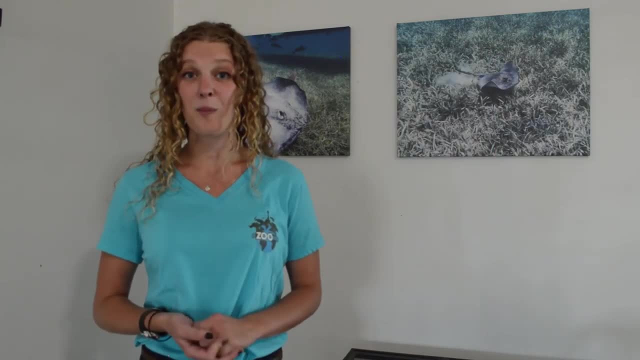 big part of their diet, But lucky for the kelp a lot of the times. there's a lot of fish that are feeding on the kelp And that's a big part of the kelp, But lucky for the kelp a lot of the times. 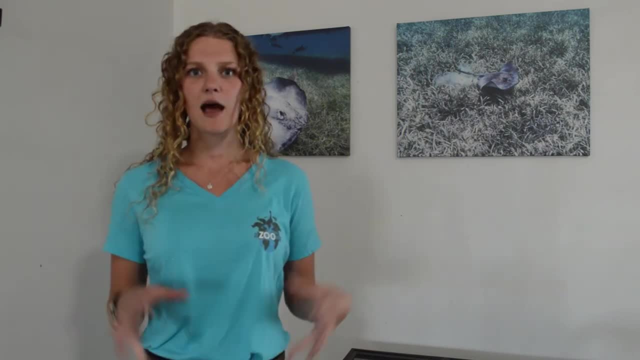 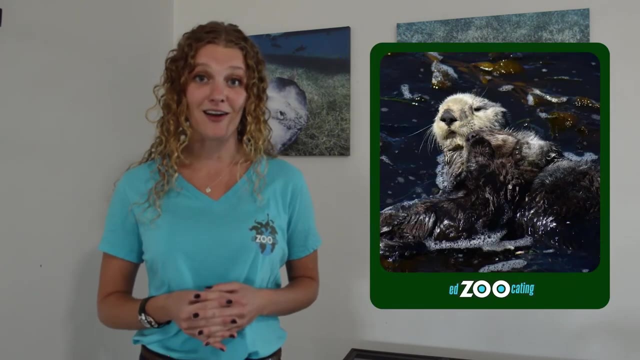 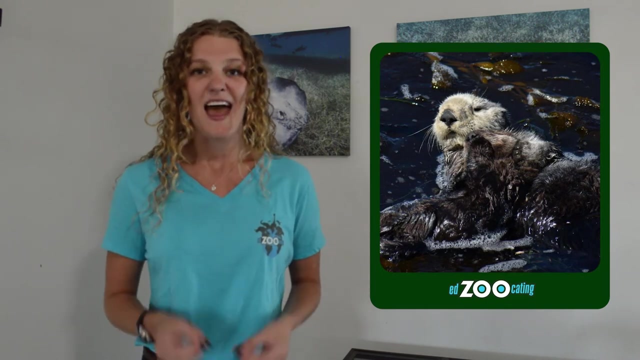 there's another animal that lives in that area that helps keep the sea urchin population under control, And that is the very cute and cuddly sea otter. They can dive way down deep to the bottom of the kelp forest where those sea urchins might be munching on the kelp. 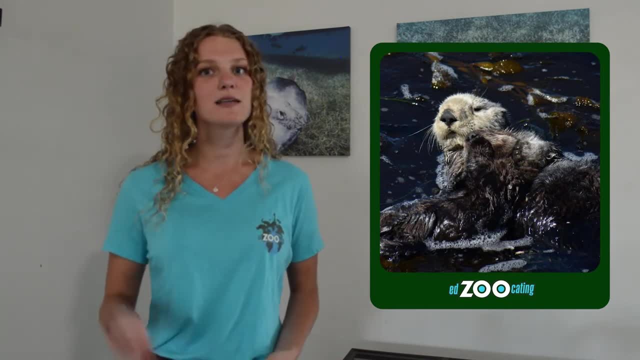 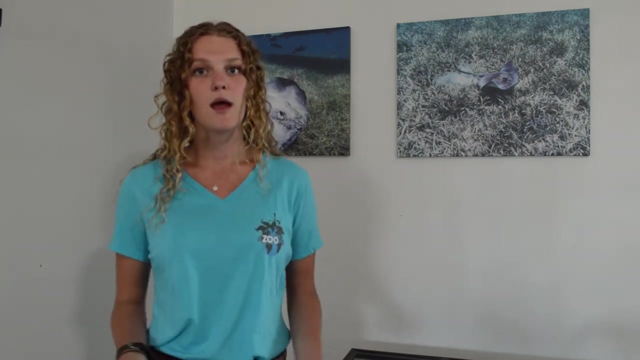 And they love to eat those sea urchins. So because we have sea otters eating the sea urchins, not that many animals are there to eat the kelp And these forests can stay nice and healthy. So all of the different animals that we find in a kelp forest have a really important role. 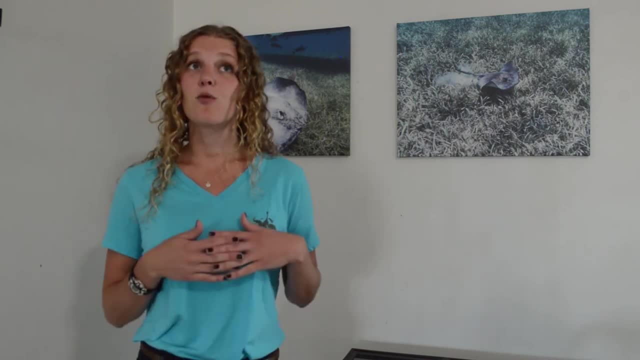 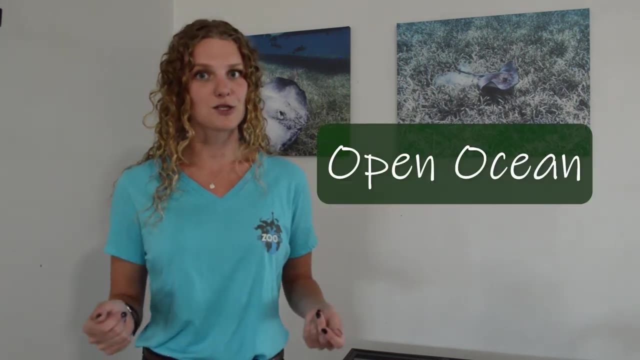 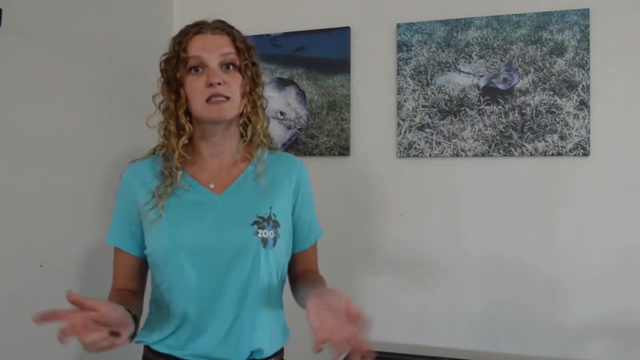 in order to keep that ecosystem healthy. And if we move beyond the kelp forest and we go even further out into the ocean, that is what we call the open ocean, And out there there is not a lot of protection. The open ocean is most of the ocean, It's. 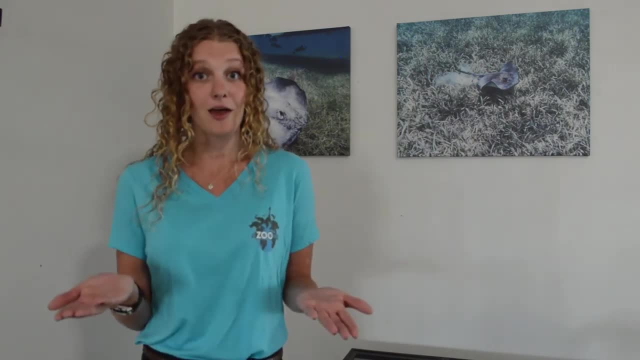 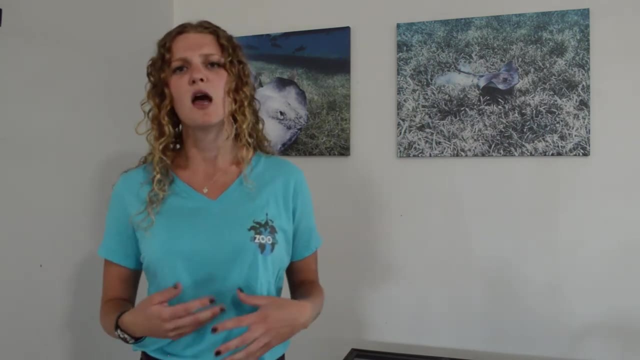 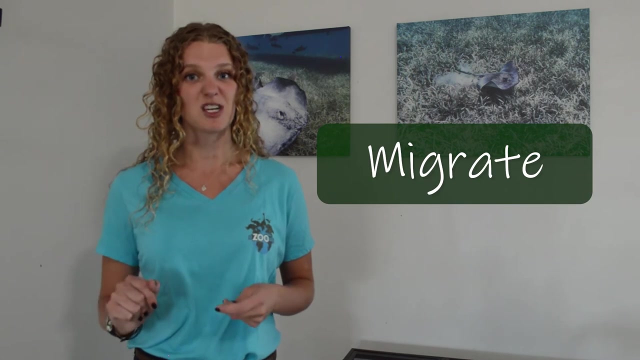 anywhere that's further away from the shore and above the ocean floor. So there's not a lot of protection, There's not a lot of water, There's not a lot of plants that grow out here. This is where we might find sea grasses over in some of the more shallow parts, But a lot of. 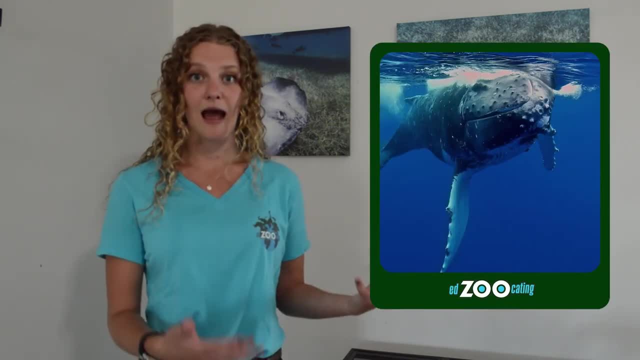 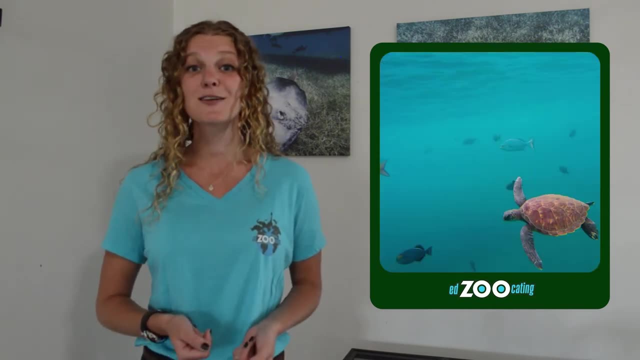 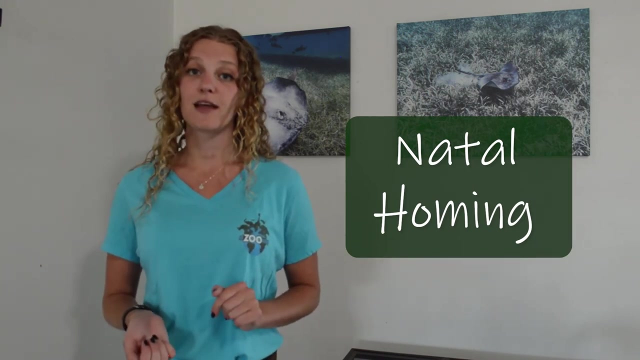 animals migrate across the open ocean. So we have whales that we said before will go to the coral reefs to have their babies. They travel great distances across the open ocean, And so do sea turtles. Sea turtles are a very cool animal. They do something that we call natal homing, which 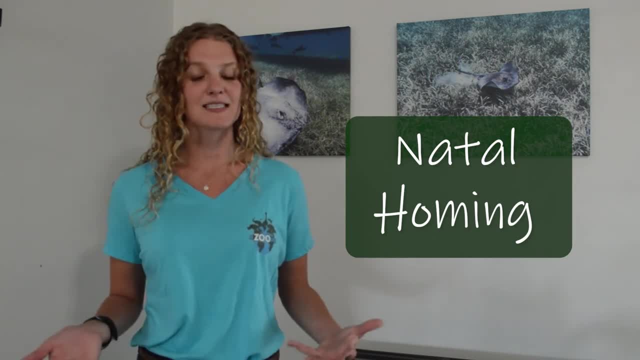 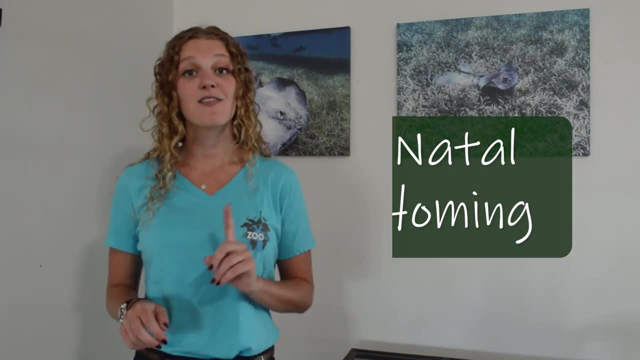 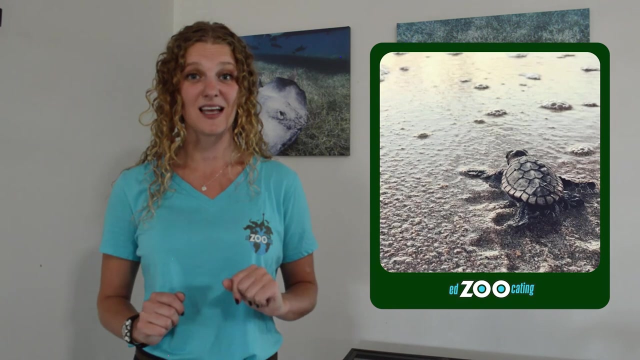 like to give things in science, And natal homing means that when a sea turtle starts out as a baby and they travel all around the ocean when it's time for them to have their babies, they travel all the way back to where they hatched And that is where they have their babies. 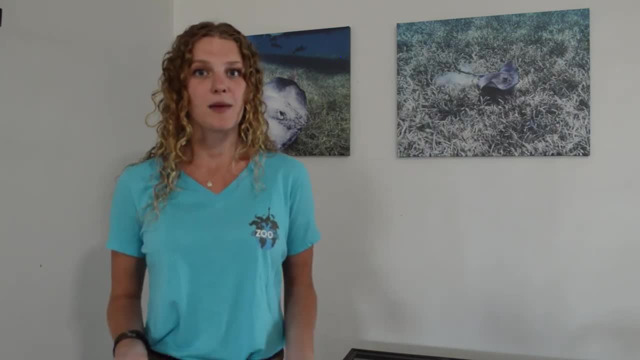 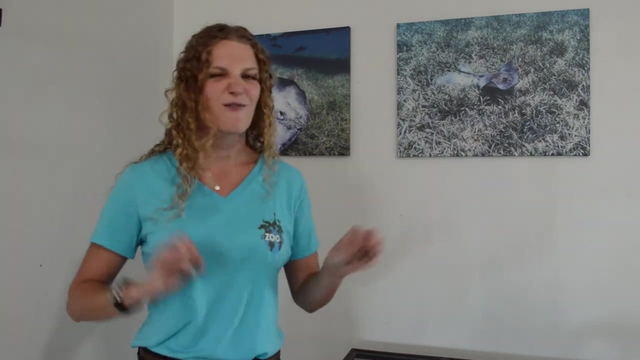 So the open ocean is a really important habitat because lots of animals need to be able to travel from one place to another. So all of these different ocean habitats are connected, And so the ocean is connected to all the different ecosystems, Just like we said. 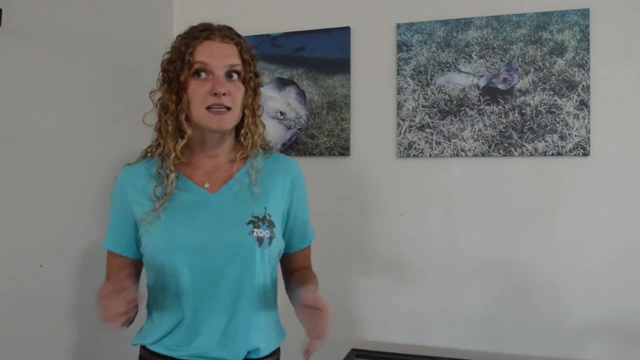 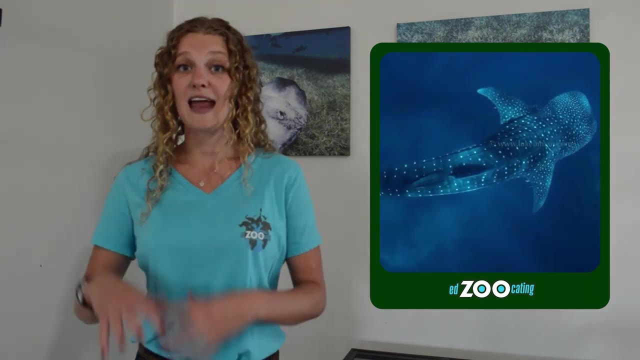 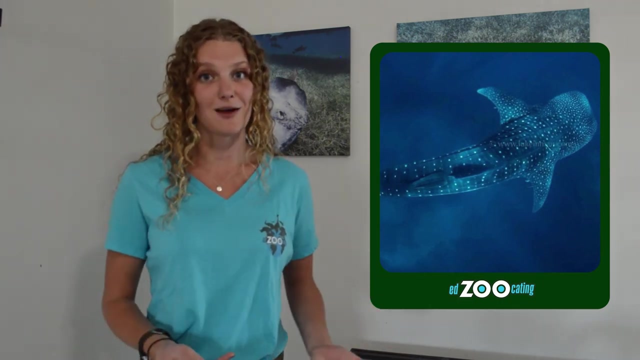 before that. all the different ecosystems are connected: The rainforest, the deserts, the ocean- they're all connected. The ocean is all connected to one another as well because of currents and animals that are migrating, So anytime we impact one part of the ocean, there is a good chance that. 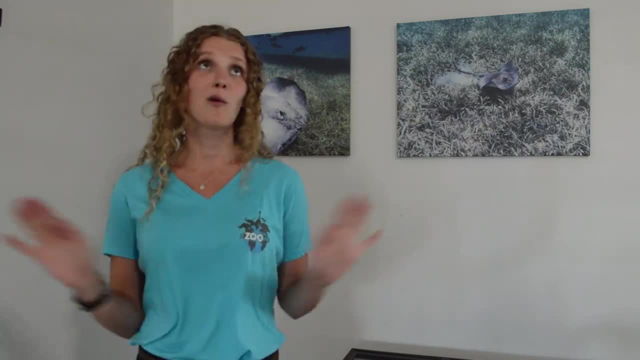 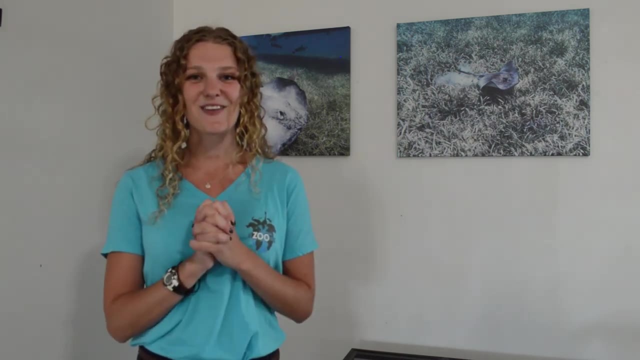 impact is going to travel and affect the rest of the ocean. So it's important that, even if you live somewhere that's in the middle of the ocean, there is a good chance that you're going to be in the middle of the ocean and you're going to be able to travel to the other side of the ocean as well. So that's why it's. 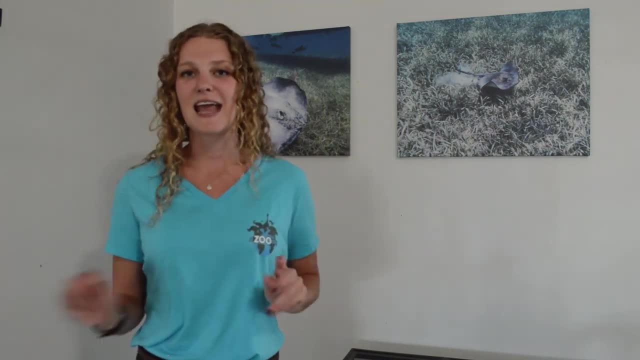 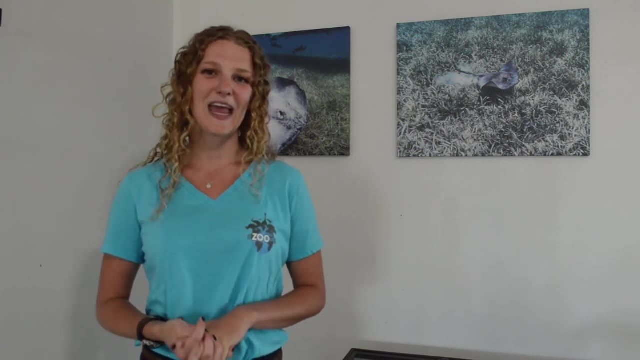 important to have a safe space in the middle of the ocean to protect our planet and our oceans. Thank you, guys, so much for hanging out with me today while we talked all about the ocean and learned the amazing biotic and abiotic factors and how they all interact with one another. And I hope we see you guys next time at our next Educating Adventure.